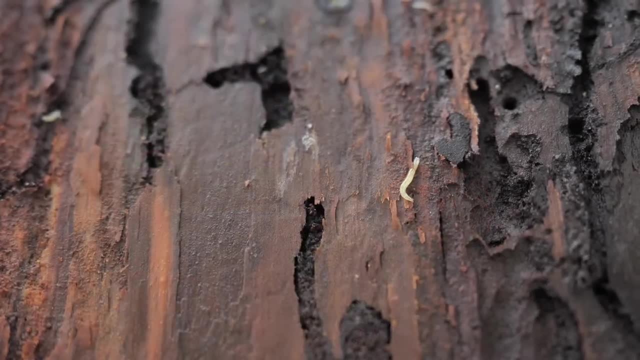 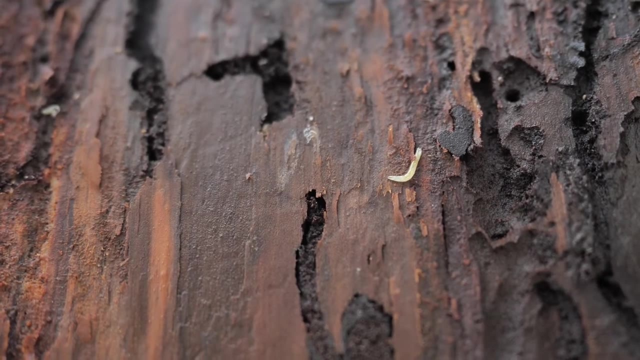 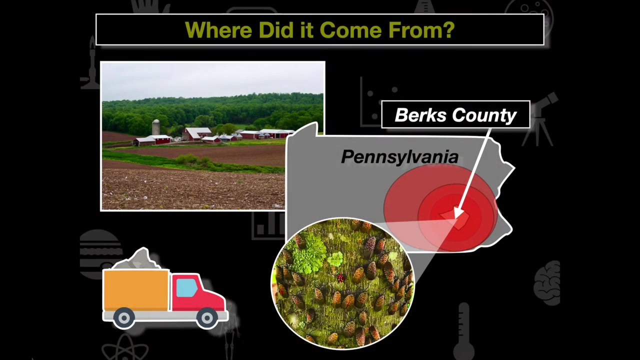 So these lanternflies have gone through and they are consuming plant material within the environments of southeastern Pennsylvania And they have been wreaking havoc on southeastern Pennsylvania because the plants and the trees that they go through and consume have no way of defending themselves And the invasive lanternflies have no natural predators. 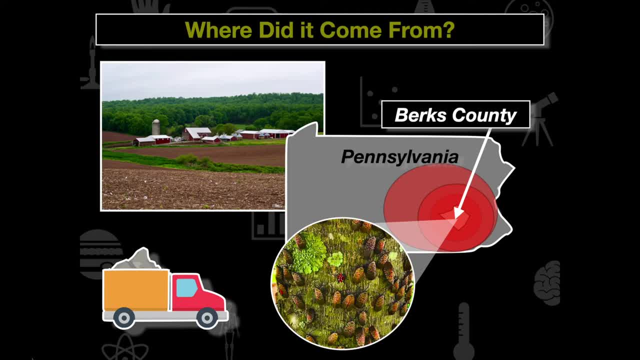 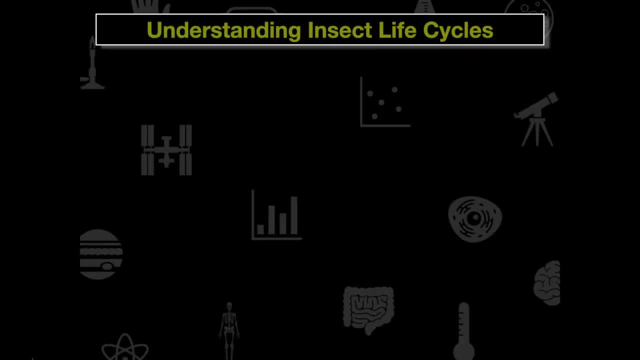 So it's important for us to understand what trees are going through and consuming and how we can prevent further degradation of the environment from this lanternfly. And in order to understand how we go through and eradicate the lanternfly, we also have to understand life cycles. 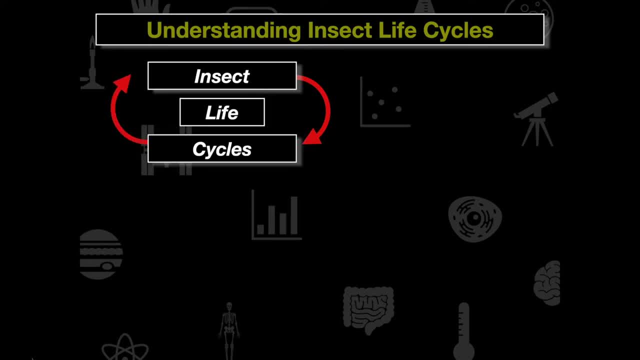 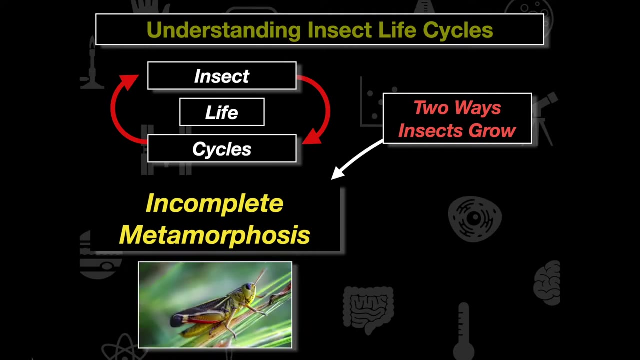 So insect life cycles go through And this is essentially how these insects go through and grow from adolescence to adulthood- And there's going to be two ways that insects mainly grow. We have incomplete metamorphosis, and that's in the case of the lanternfly and grasshoppers. 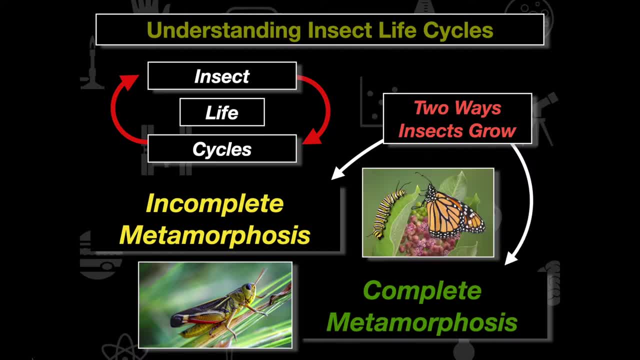 And then we're going to have complete metamorphosis, And this is something like butterflies: We go from a caterpillar to a complete butterfly here. So what we're going to do is look at these two insect life cycles. We're going to go through and study this. 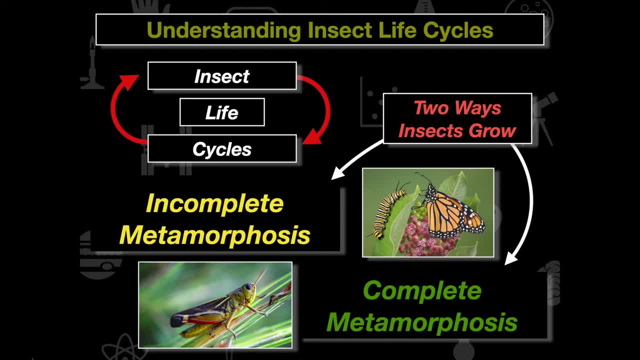 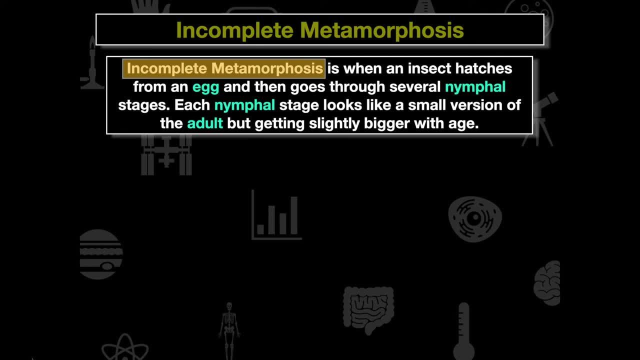 And then we're going to go through and understand How the lanternflies go through, go from their nymphal stages to the adult stage Now, in incomplete metamorphosis, this is when an insect hatches from an egg and it goes through several nymphal stages. 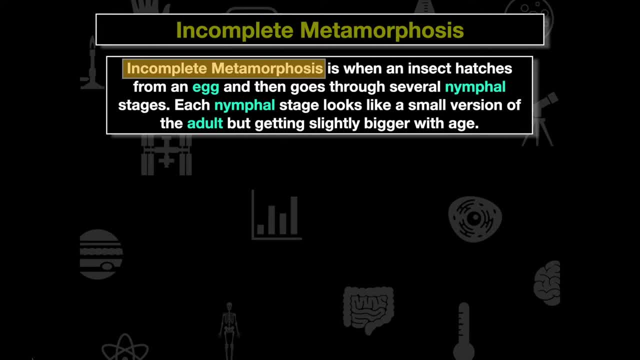 Each nymphal stage kind of looks like a smaller version of the adult, but getting slightly bigger with age. So we're going to start with the egg and we're going to look at it in the case of a grasshopper. here We're going to see what we call a nymph. 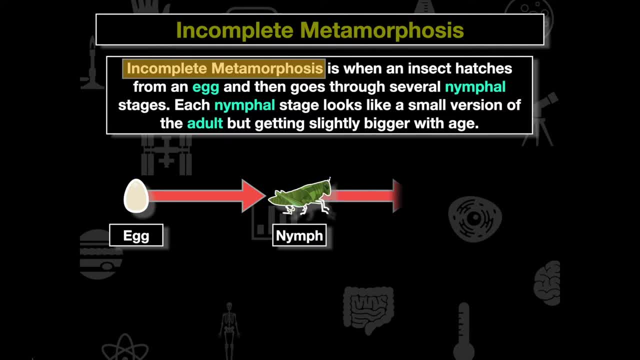 And a nymph is going to be almost like a baby insect of that full grown adult. And when we go through these stages here we go from egg to nymph to adult and then the adults go through and they lay their eggs again. So in incomplete metamorphosis- remember we call these nymphal stages when they look like a smaller version of the adult. 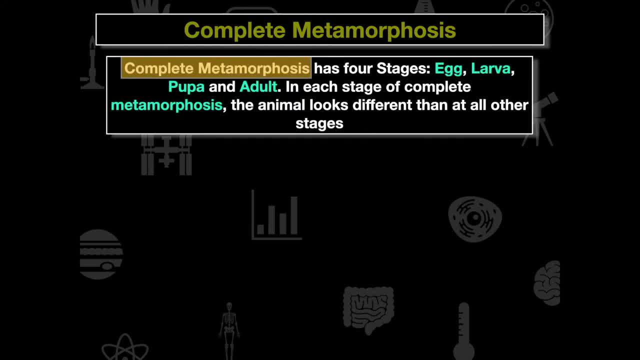 Now incomplete metamorphosis. well, this is going to look different. We have four very distinct stages: the egg, the larva, the pupa and the adult, And in each stage of complete metamorphosis the animal looks different than all other stages. 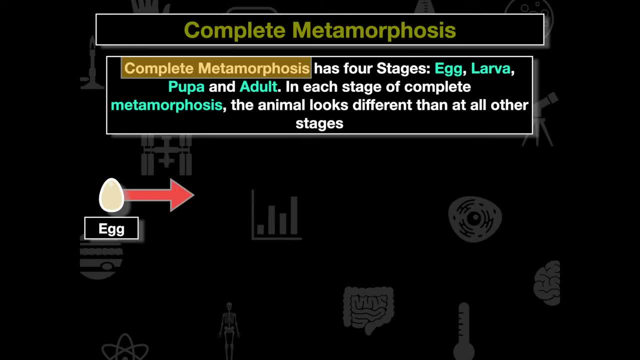 So, again, with this complete metamorphosis, we're going to start with the egg, but we're going to move into this larval stage here. This is going to be like the caterpillars that we see out in the wild. Now, as we go from here, the caterpillar is going to go through a pupa stage, where it's going to be a pupa. 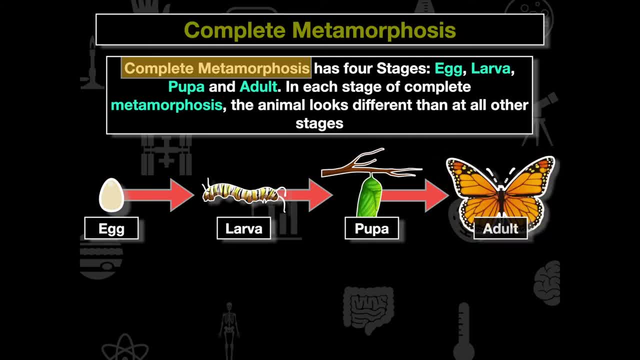 And once it goes from pupa it's going to move into its full blown adult, And the adult looks very different than the larva. And again, this life cycle- we're calling them cycles because they're going to go through, They're going to occur in a cyclical pattern, but remember, in complete metamorphosis each stage looks distinctly different. 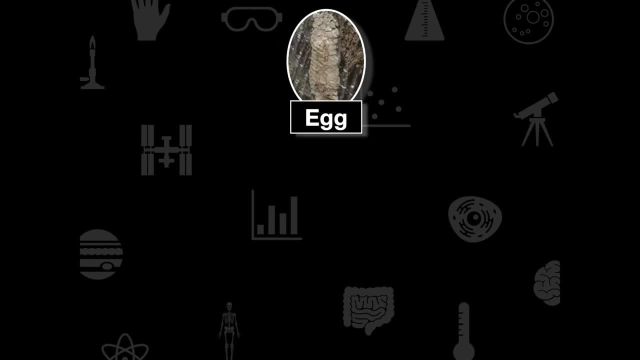 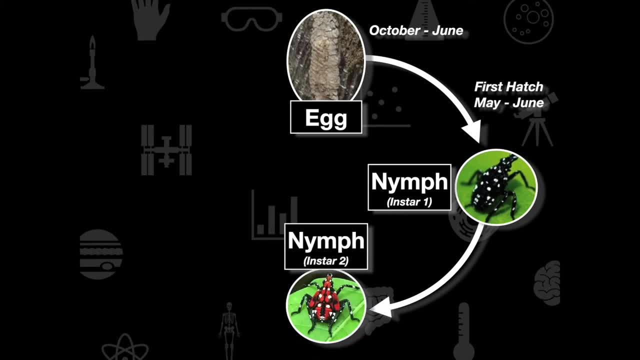 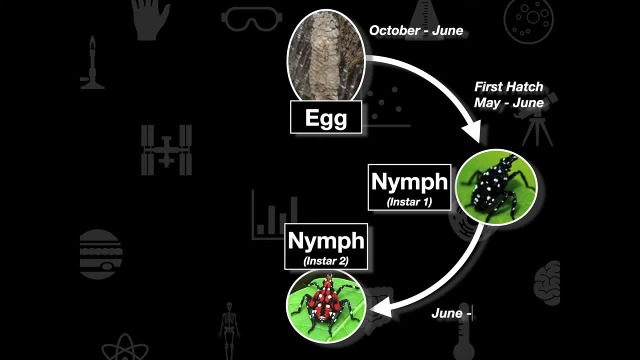 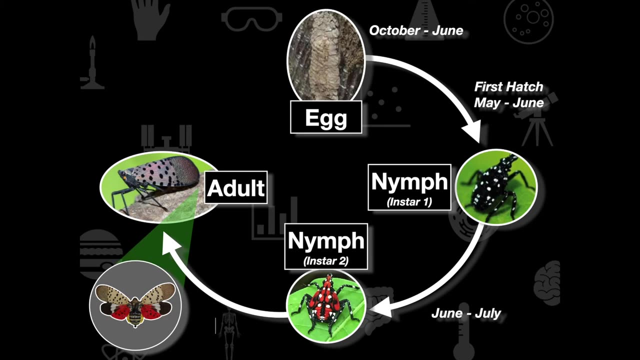 legs with a red body now and we generally see this stage from june to about july. this is the shortest stage of the life cycle. now from this in star 2 we're going to see the full-blown adult lanternfly, where the wings go through and fully develop and this adult remember. this is a pattern. 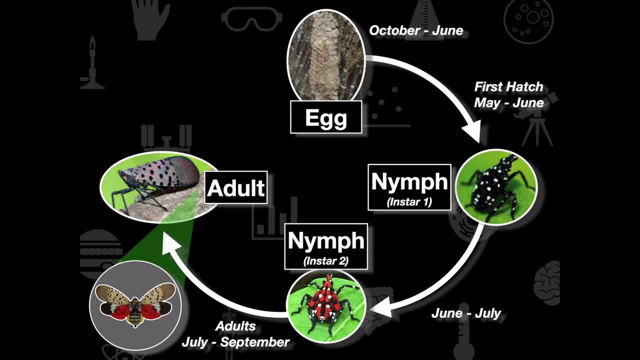 it's going to go through, develop from july to september and then it's going to go through and lay its eggs from october until you know december, and we're going to see this pattern go through and occur again. so this is going to be the incomplete metamorphosis of the lanternfly and we can see.